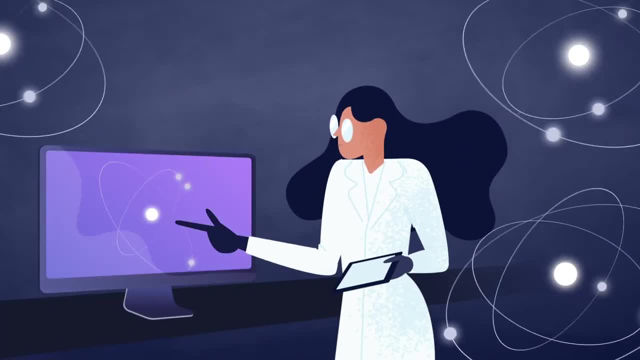 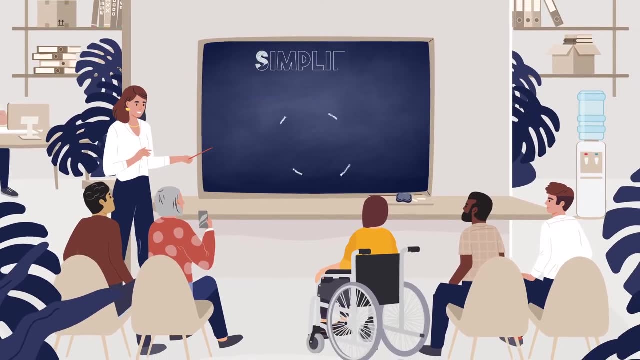 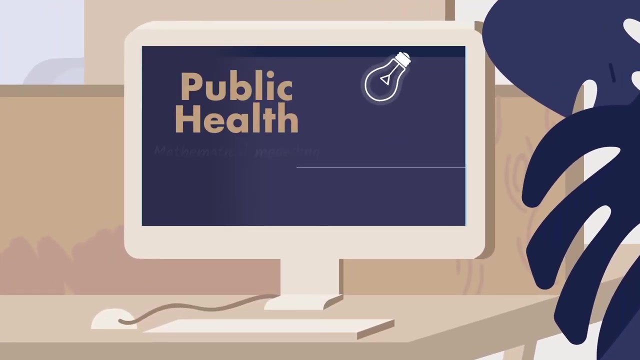 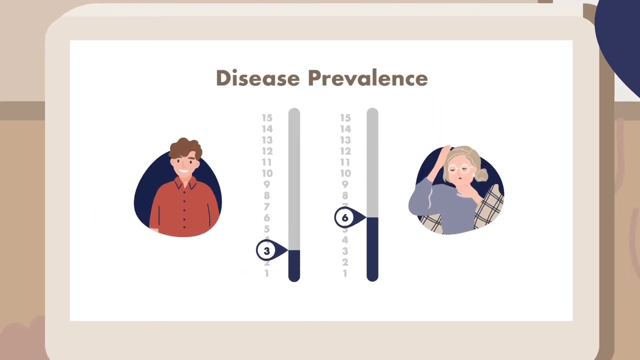 A model is a representation or simulation of something in the real world. Mathematical modeling is a research method that uses mathematics to create simplified descriptions of systems, behaviors and processes In public health. mathematical modeling is used to help answer difficult questions and understand complex relationships between biological, demographic and environmental factors. 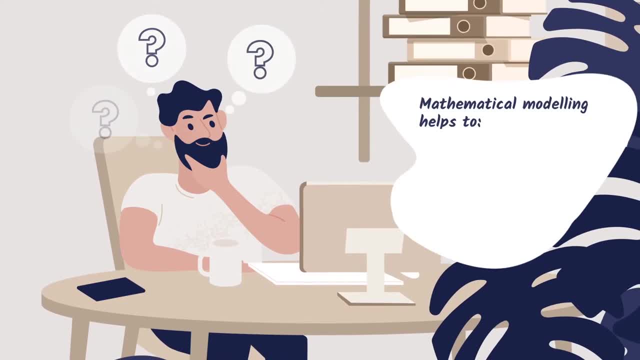 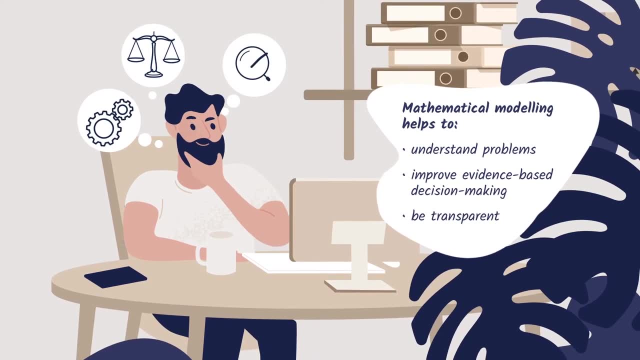 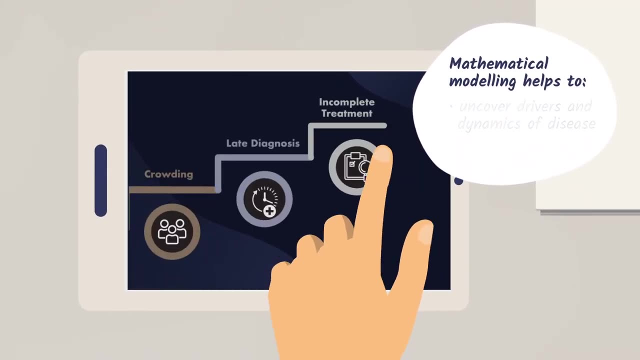 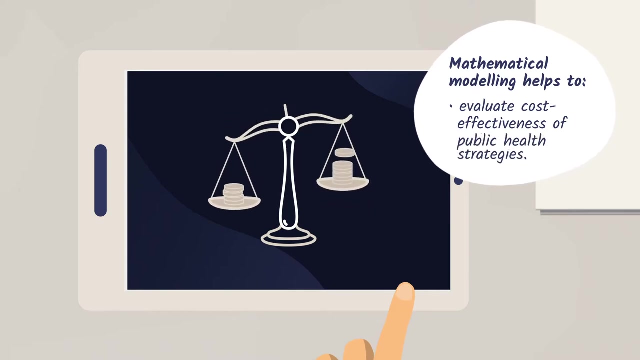 Mathematical modeling cannot answer everything, but it can be very useful to understand certain types of public health problems and improve evidence-based decision-making with transparency. For example, modeling can help uncover drivers and dynamics of disease and mortality, forecast future disease burden and intervention outcomes, and evaluate the cost effectiveness of public health strategies. 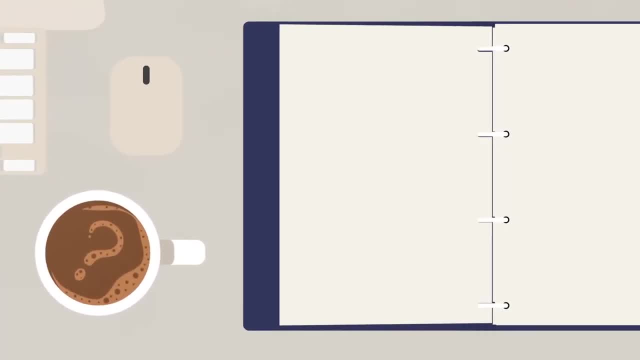 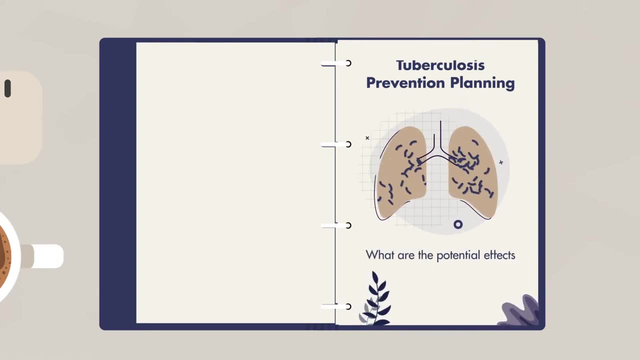 Every mathematical model begins with a question. Using tuberculosis prevention planning as an example, our research question could be: what are the potential effects of three interventions on TB incidence: One, purchasing a rapid diagnostic machine. Two, conducting regular screening in schools. Or three, improving treatment success rates with incentives and enablers? 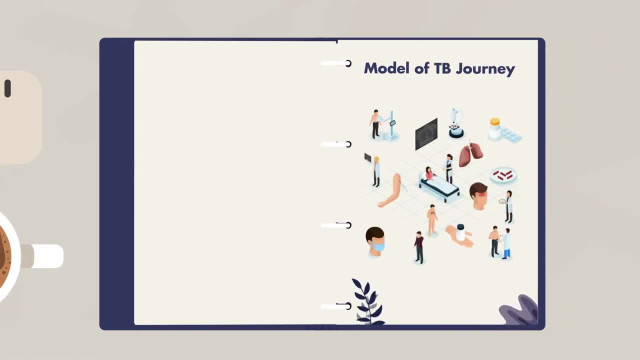 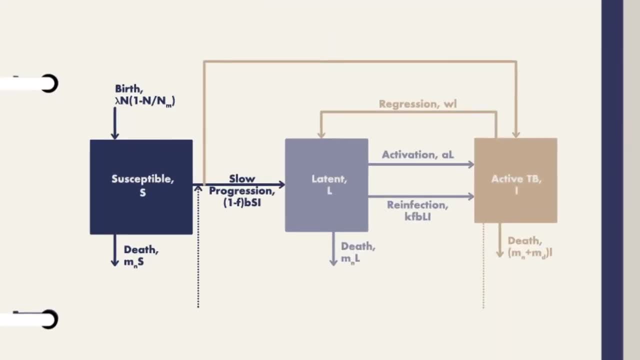 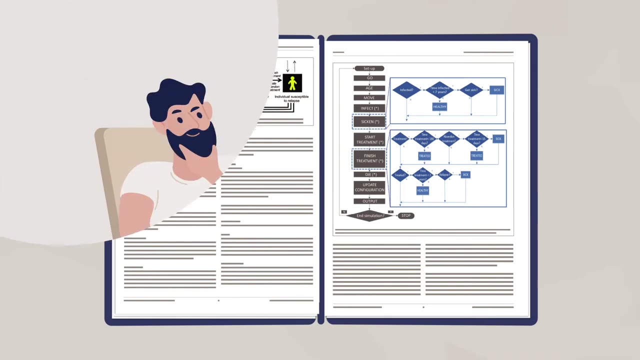 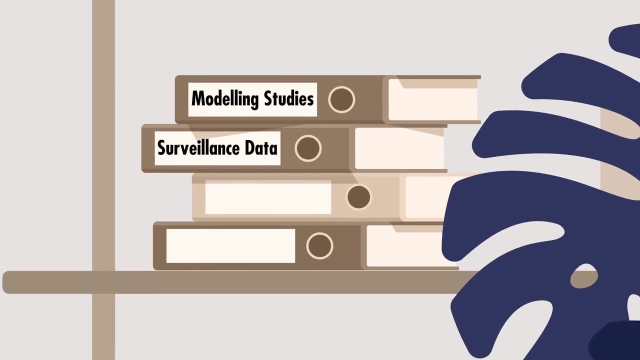 TB is a complex disease and its transmission is affected by many factors, But mathematical modeling can use what is most relevant to our question to untangle this complexity. An effective model of the world we are simulating requires gathering good information from sources like existing modeling studies, surveillance data, research papers and expert opinion. 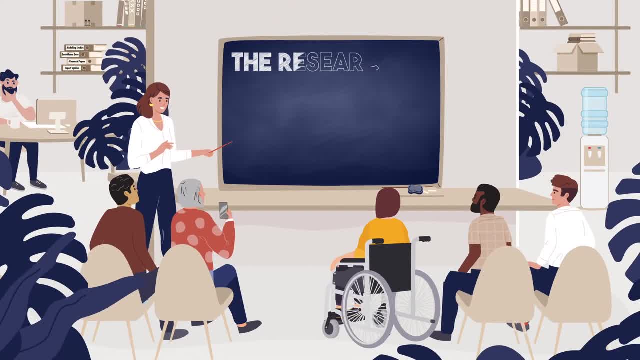 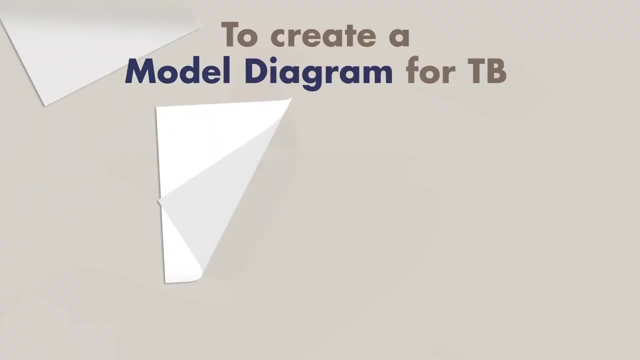 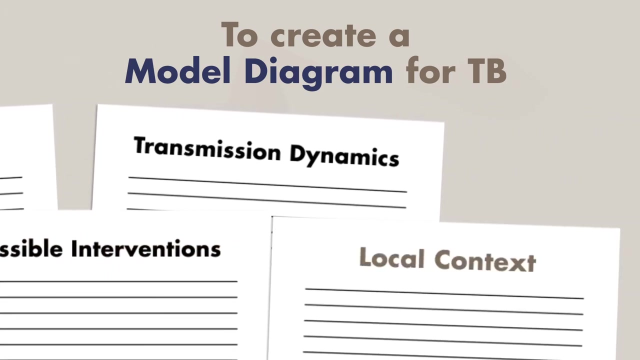 A modeler will help us decide which specific method works best for our question, For example, dynamic or static, individual or compartmental, stochastic or deterministic, cohort or transmission. Next, to create a model diagram, we will need to use what is known about TB and how it spreads, as well as information on our interventions and local context.